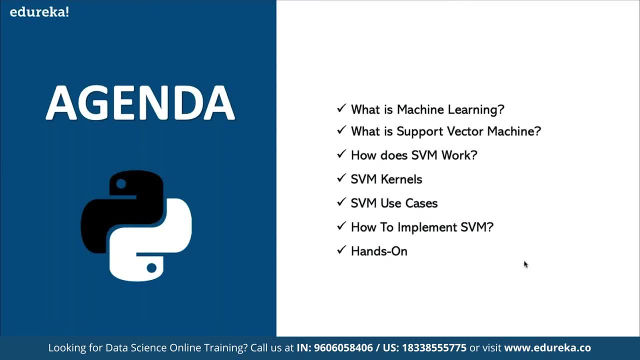 then we are going to about the components of within that process of implementation of SPM as a part of a discussion and, if time allows, and we can also see a small hands-on on top of it as well, all right. so first of all, if we talk about machine learning itself, so what exactly is machine learning? 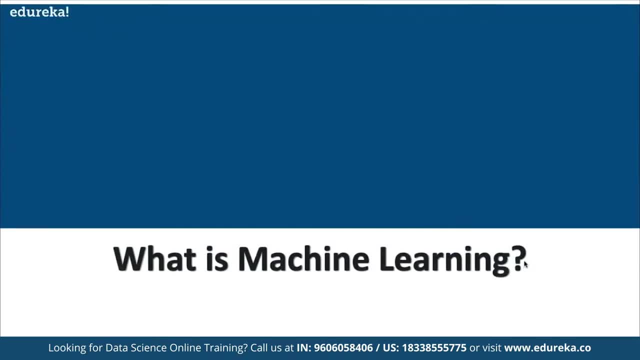 so machine learning is simply making sure that we are going to automate the entire system by using a good amount of data set right. so we can say machine learning is simply the process of feeding a machine enough data to train and predict a possible outcome using the algorithms. 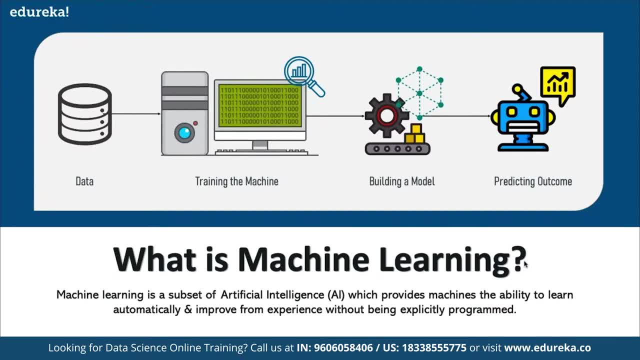 which we have the access to. so, basically, if we use more data set, then we can increase the accuracy of the results. and let's say, you may have used multiple predictions made in support before any major match, right? so in this case let's take an example for a football penalty session. so the data of previous 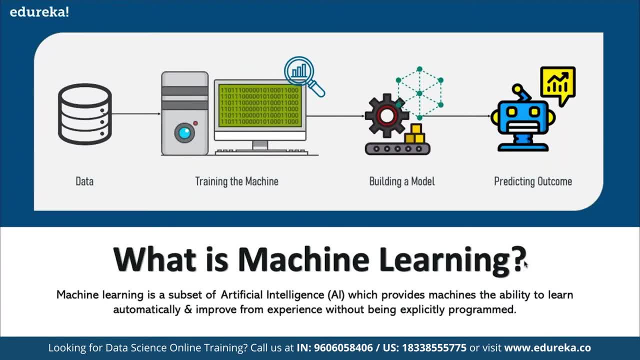 performances are going to be considered. so let's say the goalkeeper has saved all the penalties to his right in the last 50 penalties he has saved. now this data will be crucial to predicting if he or will will save or he will not save the next penalty faces. so there are other factors to 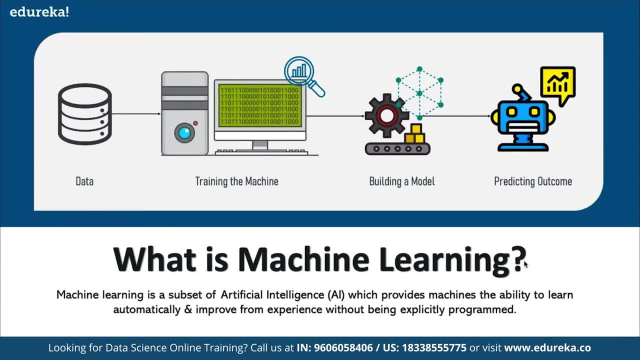 consider as well, and another example can be the suggestion that we get while surfing the internet. so the data of our previous choice is a process to give us the most favorable content we are most likely to watch. anyhow, machine learning is just feeding the machine an ample amount of data. there goes a lot of processes, algorithms and 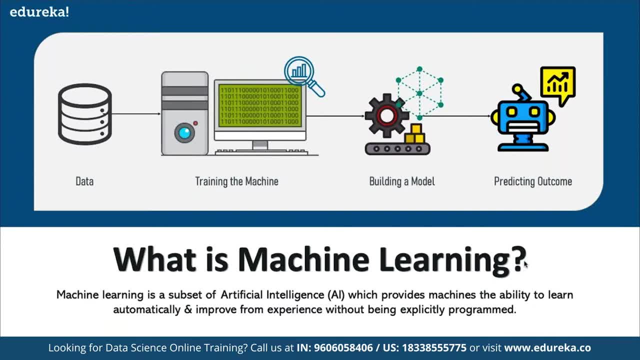 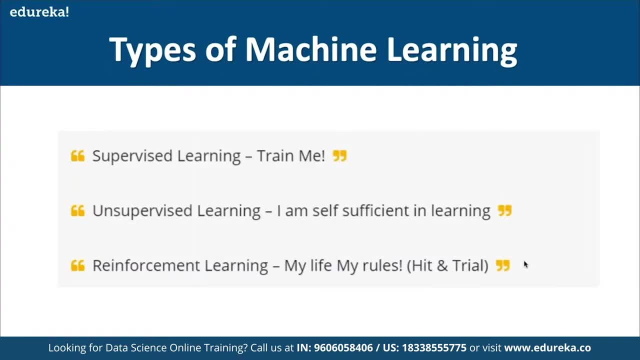 decisive factors to get the optimum results all right. so here, basically, we have three main types of machine learning as well, where we have supervised, unsupervised, and then we have reinforcement learning. so supervised, in simple terms, is: train me, it works. on a simple learning training, we have to train the model, then only it can work, and an unsupervised learning is: 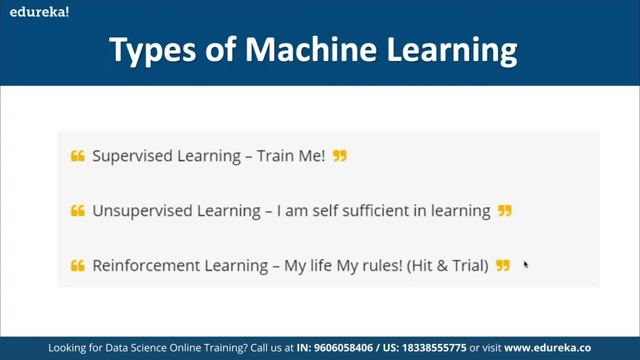 i'm sufficient. i'm self-sufficient in learning based on their own learning. we are simply going to allow them to have, we're going to allow them to have, the access as well. so that is what we are going to define for both. so, based on their own understanding, they are going to work accordingly. 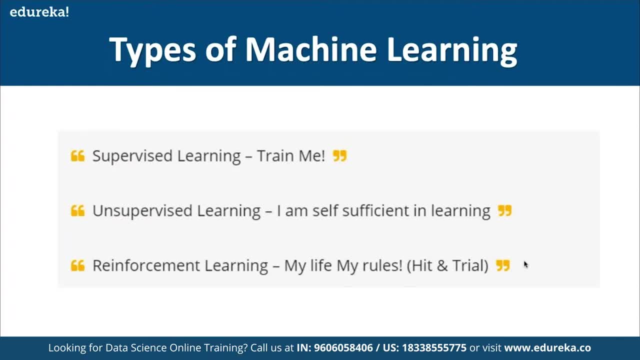 that's how it's going to work, and then we are going to work on reinforcement learning. so reinforcement learning is simply learning on its own, based on the feedback we simply trade. we simply let the system know, okay, if they have done a good job or not, and, based on that only, they simply try to get the best. 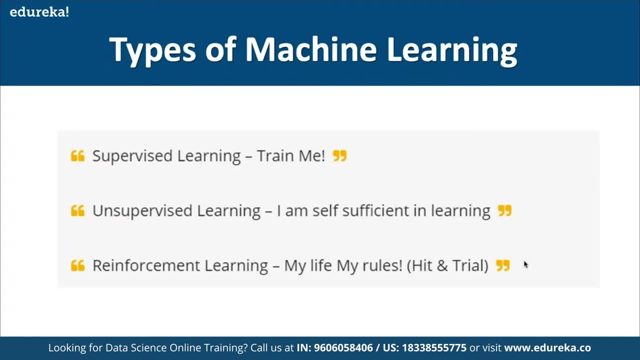 possible output. that's how it works. all right now in supervised learning we use multiple label data set to train system and under unsupervised learning we use unlabeled data set. so the data is sometimes unlabeled or we can say uncategorized, and the machine makes the best, the best possible reference. 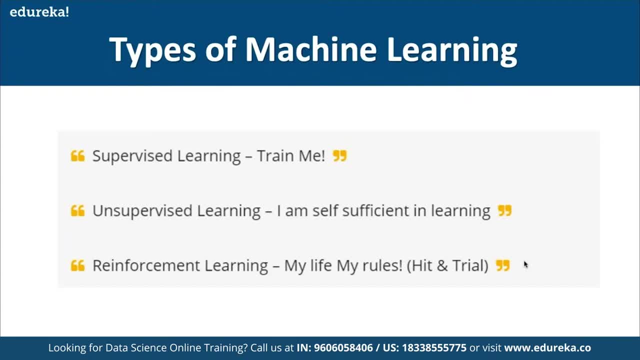 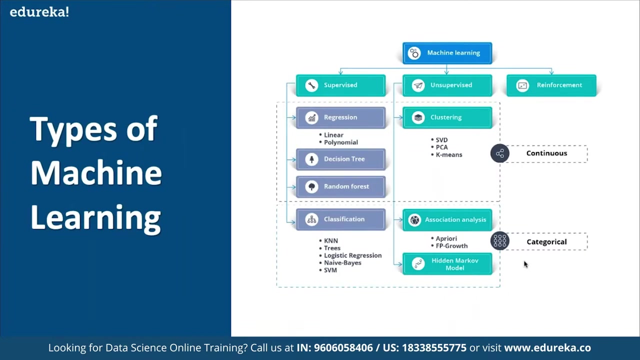 and then we have reinforcement learning. so reinforcement learning simply ensures: okay, we are simply going to create a system based on the feedback, so the machine needs to establish a systematic pattern of approach and reinforcement learning here. so that's how we discuss again here we have supervised, again under supervised. we have multiple models, like we have regression. 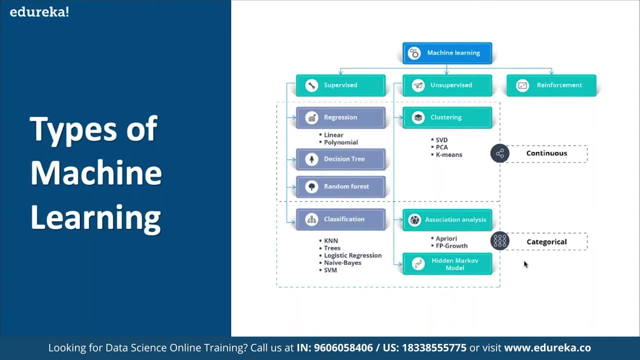 decision tree. we have reinforcement models. we have different models currently available as in under unsupervised. we have multiple models, like we have clustering. we have association analysis, we have hidden markup model. so again, the knn trees, logistic regression, logistic regression, knife base and svm. they all are types of classification where, if we talk about the 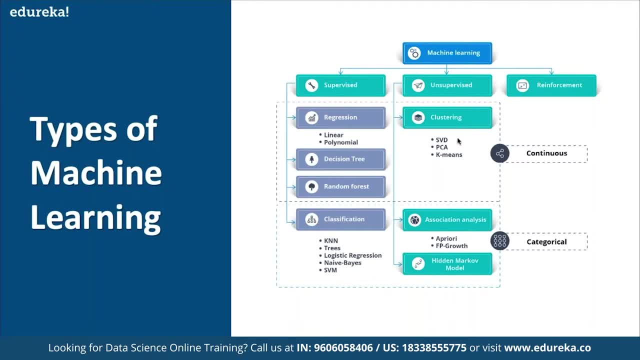 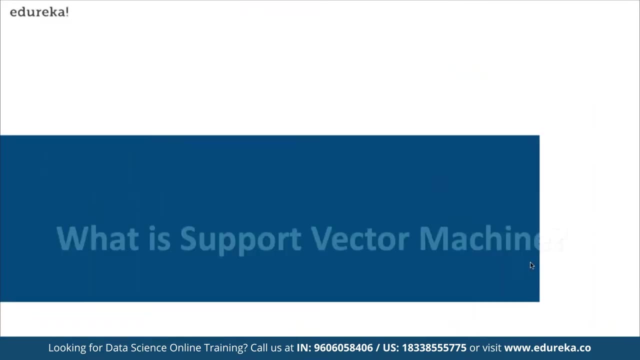 upper theory, fv growth, k means pca, svd. they all are part of unsupervised and again- reinforcement simply based on its own structure that we are going to discuss as we proceed further step by step. all right, so now next is we are going to discuss on what exactly we mean by support vector machine. 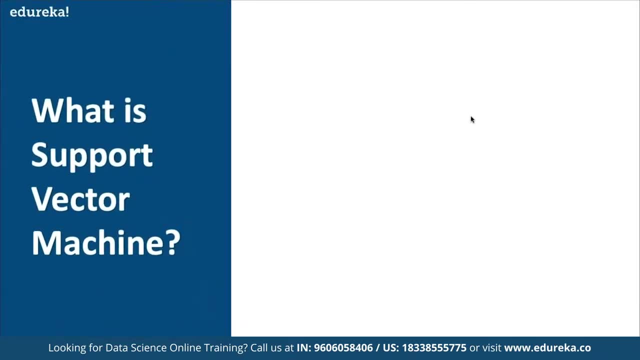 so a support vector machine was first introduced in the 1960s and later improvised in 1990s as well, and it is basically a supervised learning machine classification algorithm that has become extremely popular nowadays because of its- you can say- efficient results, and especially for the complicated. 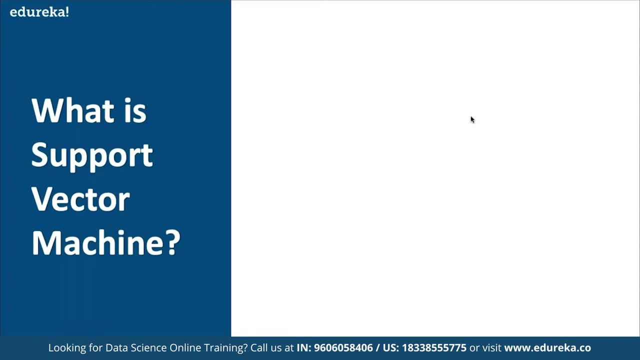 scenarios. it can deliver it for us as a part of support vector machine. as you can see here again, it's simply just like a discriminative classifier that is formally designed by a separative hyperplane itself, and svm is implemented in a slightly different way than the other machine learning. 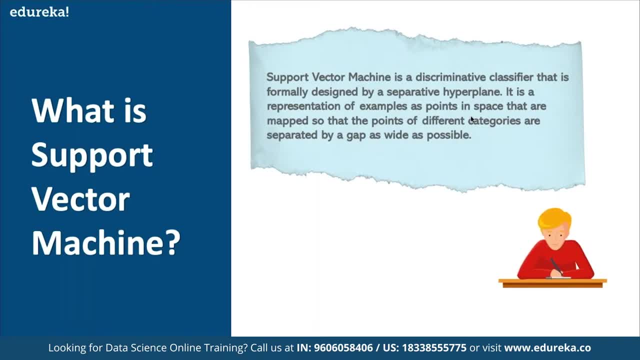 algorithms, so it is capable of performing classification, regression and outline direction as well. and support vector machine is basically again simply designed by the separative hyperplane. so basically here we can have multiple data pointers that can be mapped, so that the points of different categories are going to be separated by a gap, and in addition. so basically svm can also. 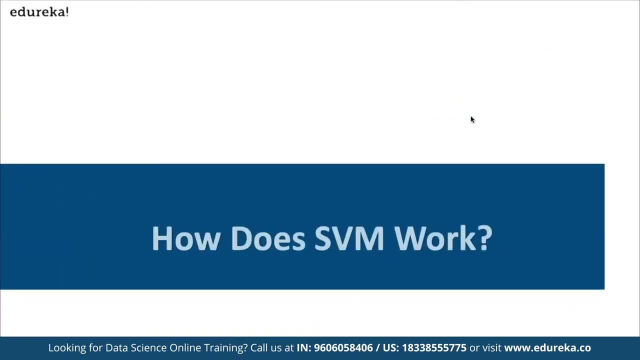 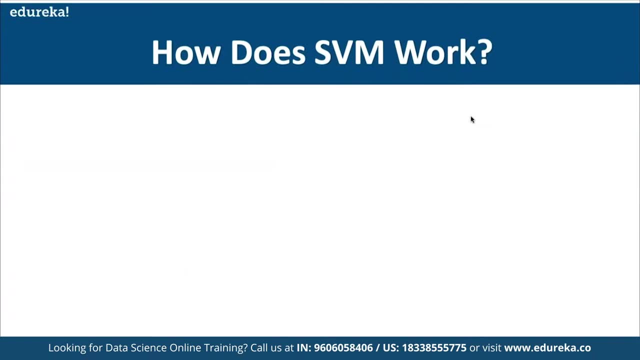 perform non-linear classification. so we'll be talking more about the how exactly support vector machine works as we proceed further. but there are multiple advantages of using svm as well. for example, it is effective in high dimensional spaces, it is effective in cases where the number of dimensions in greater is greater than the number of samples, and it is okay, it simply uses. 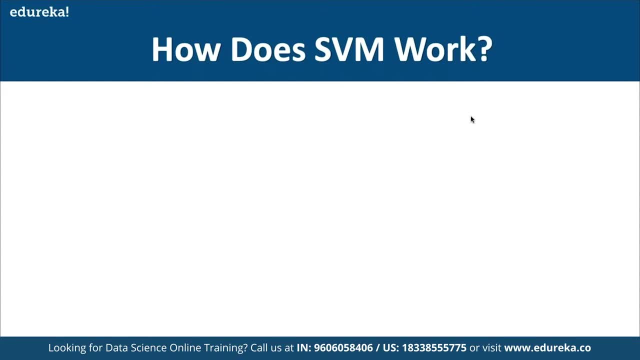 a subset of trading points in decision function. that makes it memory efficient. and it has different kernel functions that can be specified for decision function. that also makes it versatile. and same way we also have multiple. we can say downside or we can say disadvantages of using svm as well. so the number of features is much larger than the number of samples. then we 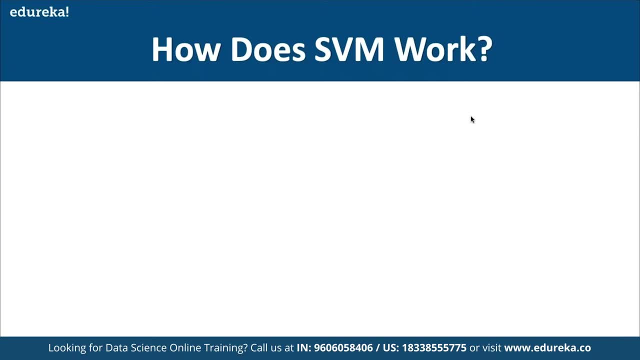 can simply avoid overfitting and choosing kernel functions. and again, recognizing them is crucial. and svm did not directly provide probability estimates and these are calculated using the five-fold cross validation. and how does svm work? so the main objective of a support vector machine is to segregate their given data in the best possible way and when. the segregation. 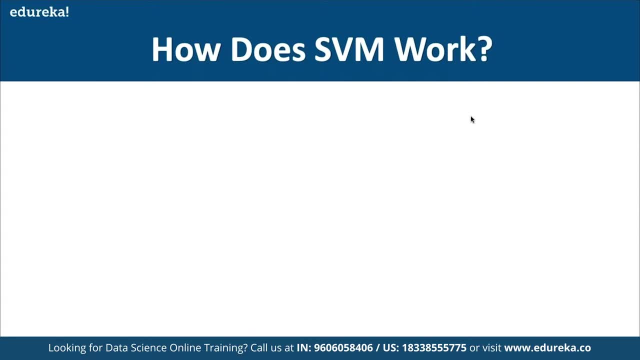 is done, the distance between nearest point is known as the margin, and the approach is set to a hyper, basically hyper- plane with the maximum possible margin in the support vector, as we can see here. that has been right now presented all right, and now basically here to select the maximum hyperplane. 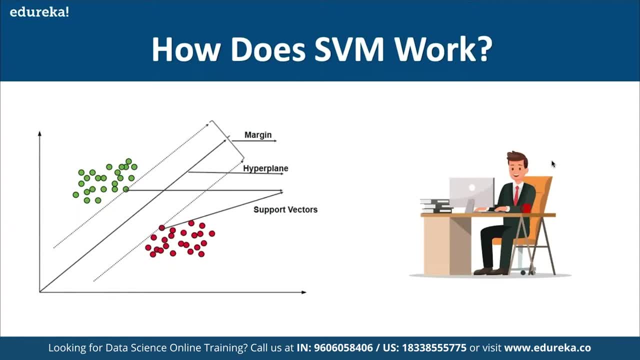 so now here in the given sets, the support vector machine follows again multiple sets. for example, it's simply going to generate the hyperplane which segregates the class of the classes in the best possible way, and then we are going to select the right hyperplane with the maximum segregation from either nearest data pointers. so basically there, 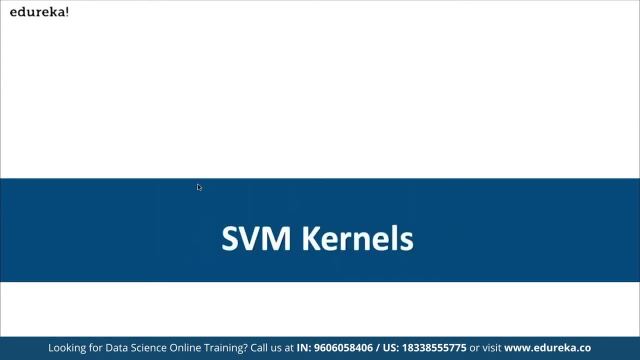 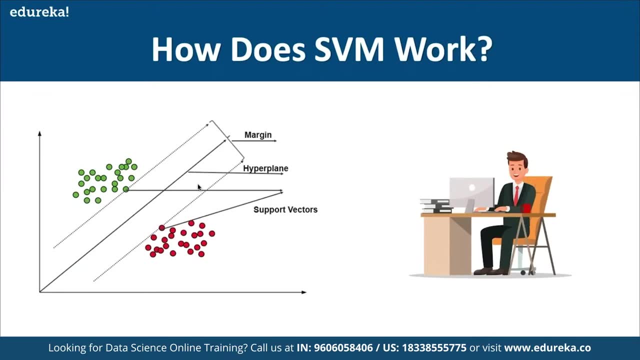 are different ways of or even dealing with inseparable or, we can say, non-linear planes as well. so, for example, in some cases hyperplanes cannot be very efficient and in those cases the support vector machine uses a kernel tick from a kernel trick to transform the input. 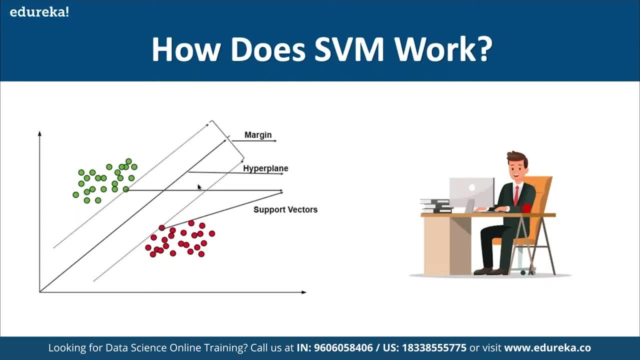 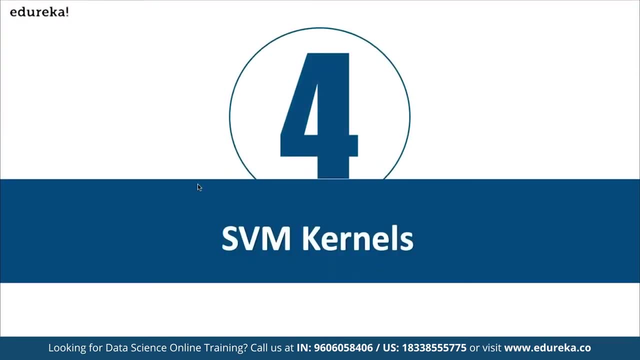 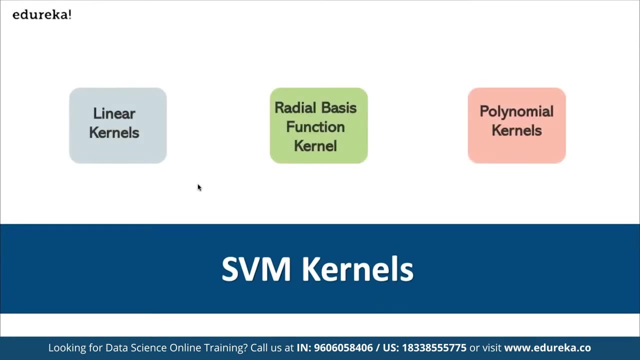 into a higher dimensional space and with this it becomes easier to segregate the pointers. so now let's talk about the svm kernels. so basically, svm kernel adds more dimension to a lower dimensional space to make it easier to segregate the data. it converts, the inseparable 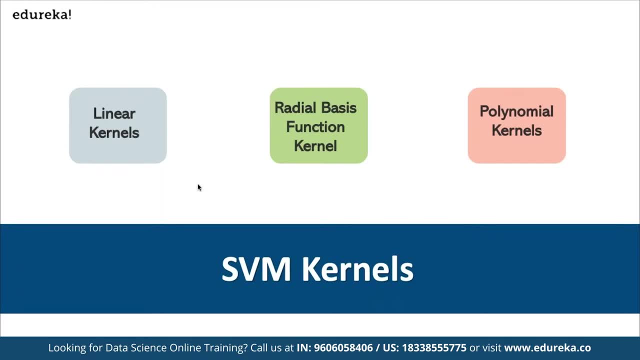 problem to separable problems by adding more dimensions using the kernel trick and a support vector. machine is implemented in practice by a kernel, and the kernel and the kernel is decomposed. the волker 드 Соps hat theomics are created electronically. that's howess applied after they 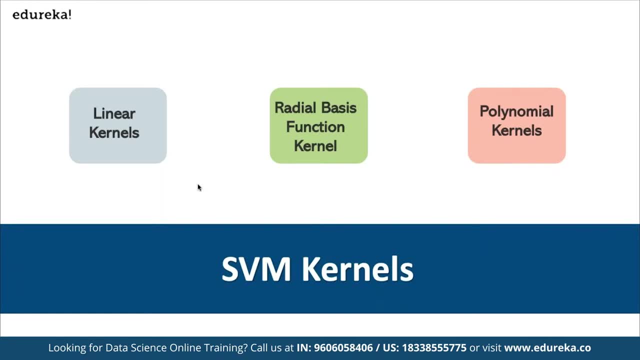 have been pulled off because it's morelogical gas by moving on september. in 2017, there are much moreMusic wands. the kernel trick helps to make more accurate classifier so we can take a look at different kernels in a support vector machine, like we have linear, we have radial base and then we have 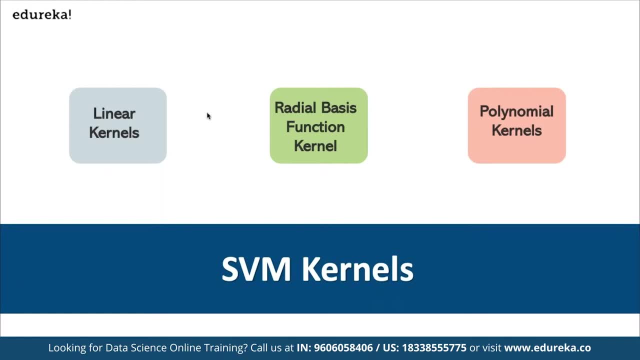 polynomial kernels as well. all right, and so a leader kernel can be used to as a normal dot product between any two given observations. so the product between the two vectors is the sum of multiplication of each pair of input values. so we can understand this for a simple limit example as well. so if we talk about the linear kernel, so basically, as we, as we, 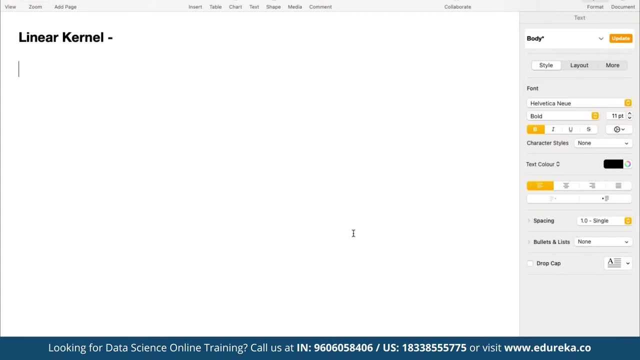 discussed linear kernel can be used as normal dot product between any two given observations. for example, here we can find this one as opposed to zero, and it can be added to so of, let's suppose, multiplied by x, xi. all right, so as we discussed again here, it is going to be the 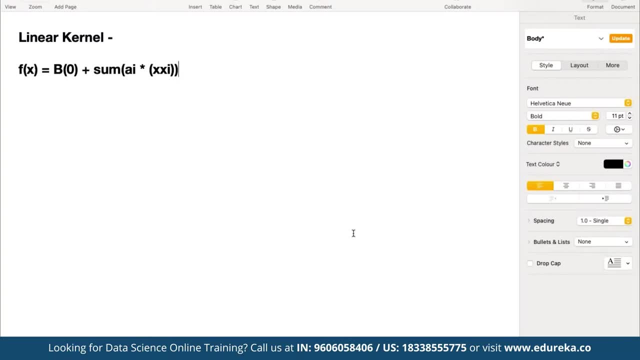 product between two vectors is the sum of multiplication of each pair of input values as a part of simple linear kernel equation. and then we have polynomial, so this one is for linear kernel, then we have for polynomial kernel, so polynomial kernel is what polynomial kernel is like, a it's rather generalized form of the linear control and again it can distinguish. 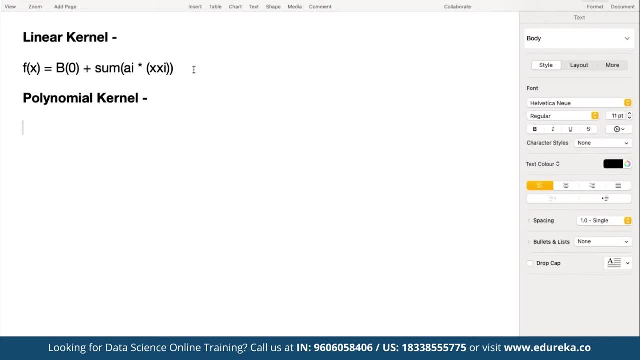 curved or non-linear input space. so for example, here we can refer this as opposed as k, and then we can define multiple pointers, i suppose x, 1, x 2, and then we can simply add this to a point, and then we can simply add this to a point, and then we can simply add this to a point, and then 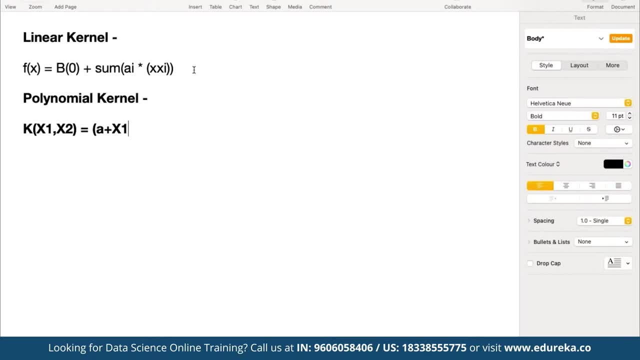 because now here we have defined, suppose, x 1, and again all the clicker defined here x 20, and then x 1, 4, again this value for x 2, here for x 2, and again the entire one has to be raised to power. 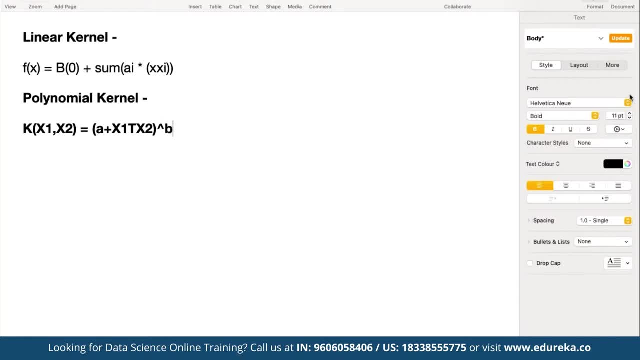 b itself just a moment. so next we, after polynomial, we are going to have- we also have radius space. so here, after polynomial, we have the radial basis function kernel. so in terms of radial basis function kernel, so here the radial basis function kernel is commonly used in the svm classification and it can map. 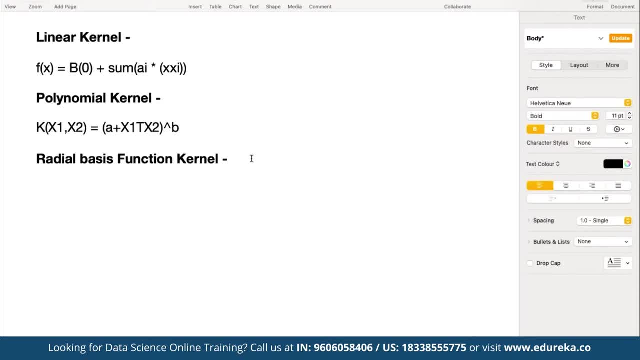 the space in infinite dimensions. so basically, if we talk about the actual dimensions here, so here we can represent it as suppose the value of k, x1, and again for x2, and here we can find the exponent where expert is going to be, suppose for minus 4. 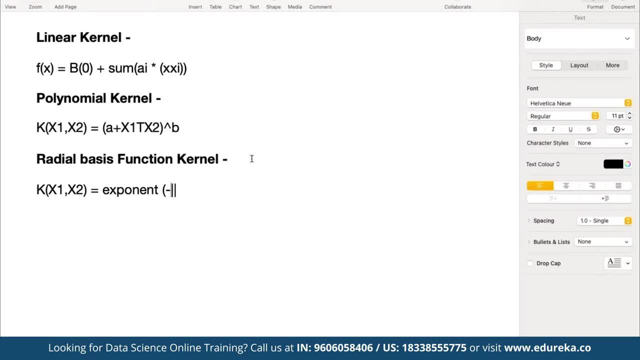 again the gamma value, and let's say we represent this as y and then we can define this for x1 minus. this is going to be x2, and then it has to be raised to power 2.. so basically, x1 minus x2 is simply going to be 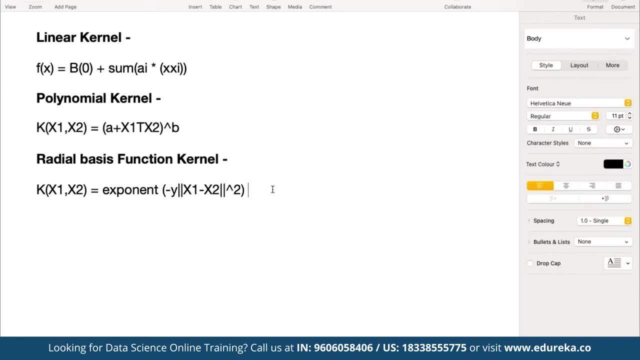 the euclidean distance between the x1 and x2. so we can say x1 minus x2 is euclidean distance, is the euclidean distance between x1 and x2, here and where, if we talk about here, if we talk about the current component for b. so here we can say: b is what b is, b is the degree of kernel. 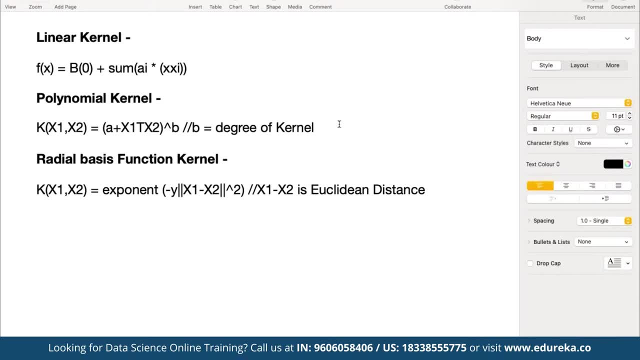 in case you don't have, we can, in case you don't have the knowledge of of it yet, and then a is going to be. or you can say: a is what a is. the constant term is the constant term that we have. so here we have linear polynomial and then we have radial basis function. so there are multiple use cases. so before 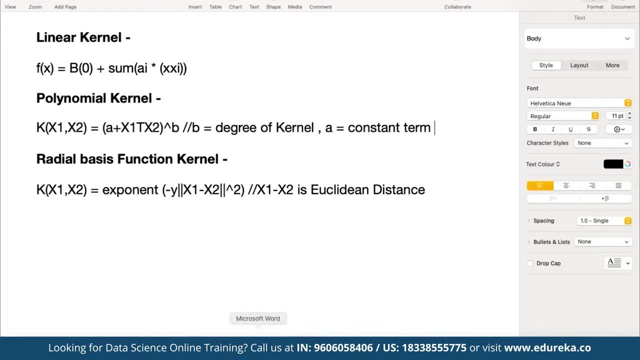 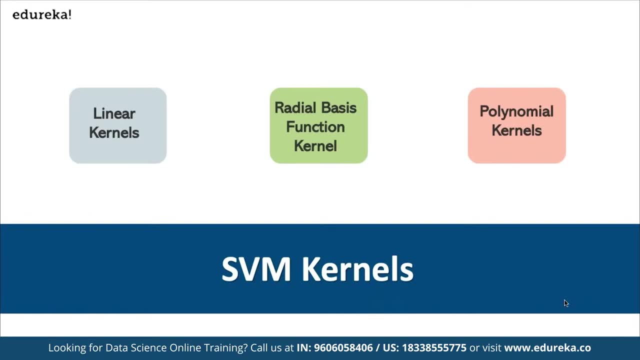 we proceed further. so there are multiple use cases of the serial base convert. I can say component as well. so here we can use it for the phase direction, for text and hypertext categorization. here we use it for the classification of images, for bioinformatics, for protein fold and remote. 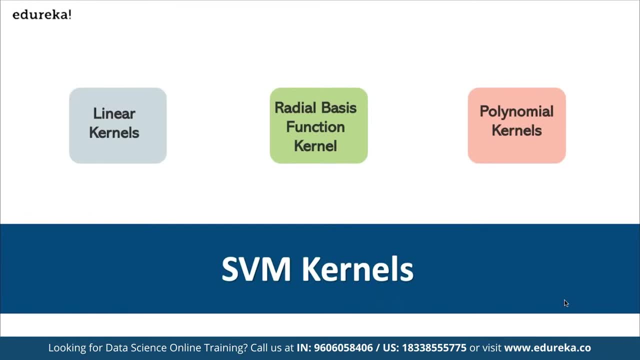 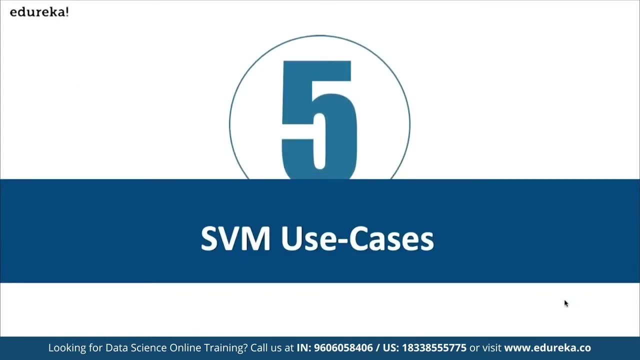 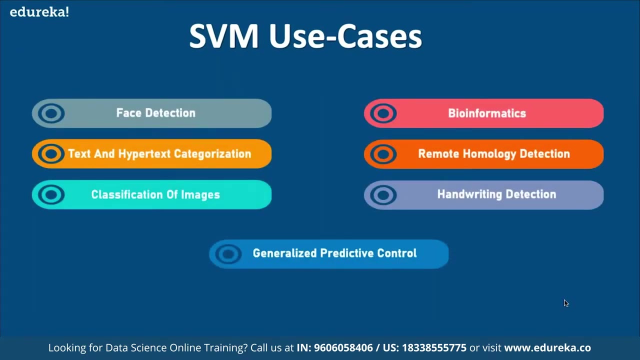 homology direction as well. we can use it for different use cases and we can also use for, again, having a prediction control as well, as we discuss in svm. so there are multiple use cases for face selection, for bioinformatics, for text and hypertext categorization for remote homology. so these are 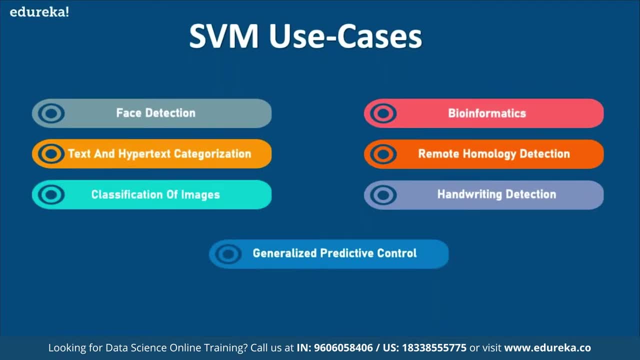 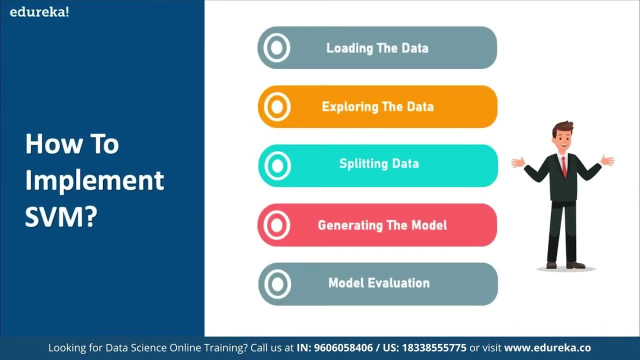 different use cases are currently available here. so now, in terms of how to implement svm. so first of all, we have to load the data, we have to explore the data, we have to split the data, and then we also have to, we also have to generate the model, and then we have to evaluate the model as well. all 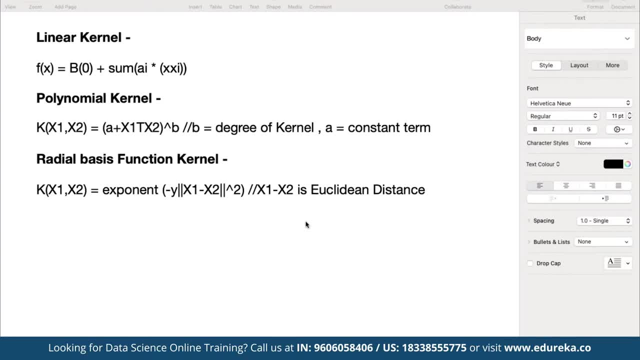 right, as we have discussed again, in case we have been confused. so linear is simply going to be the dot product between the any two given observation itself, and here we define two. here the product is going to be between two different vectors. it's simply going to be the sum of multiplication of. 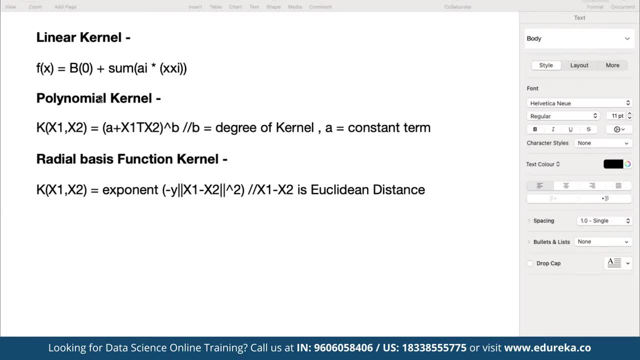 each pair and then under polynomial. so basically, here we can distinguish curved or non-linear input space where we have defined the k1 as x1, x2, for where a is where a is simply going to be a constant term and b the power to which we have increases, so b is simply going to be the degree of penalty. 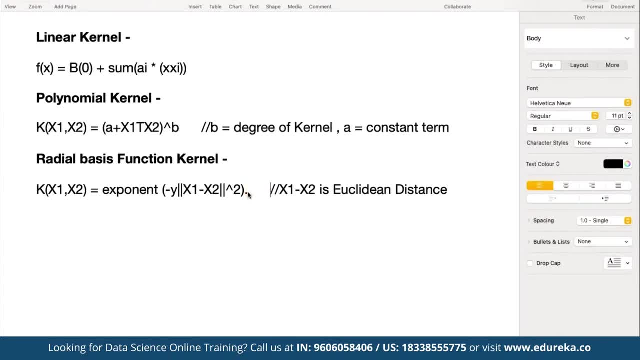 are going to make use of, and then under radial basis, as we discussed. it is commonly used in classification and can map the space in infinite dimensions as well, where x1 minus x2 is simply going to be the euclidean distance, and we can say this one. 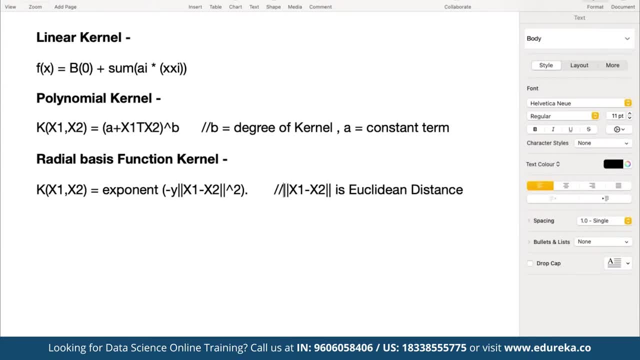 that we define here. x1 minus x2 here is simply going to be the euclidean distance here. all right, so let's do one thing: let's open up pycharm community here so we can start by a simple loading the data set and then working on top of it. 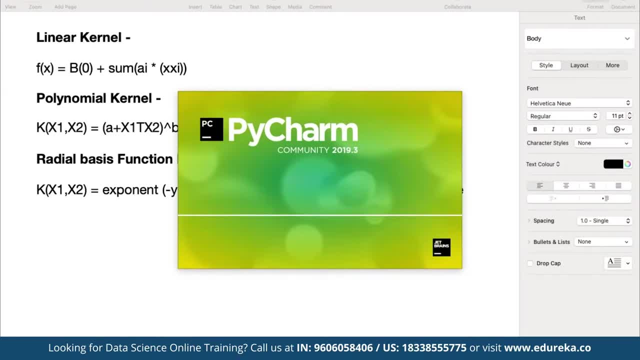 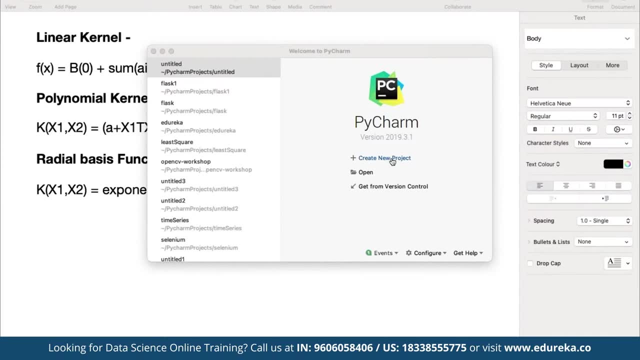 so we can use any id. we can use any python id to get started. we can use anything. so let's do one thing. let's create a new project. let's say we name it as svm, so in case you don't have the access to svm as of now, so you can go ahead and 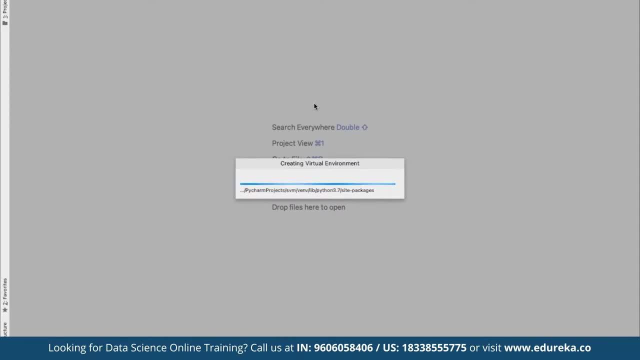 download the community version. so this is going to give you the access to pycharm, or we can use any id as well, if required. all right, so here, once we enter the project here, we can simply go ahead and create a new file altogether. so let's name it as our demo file. 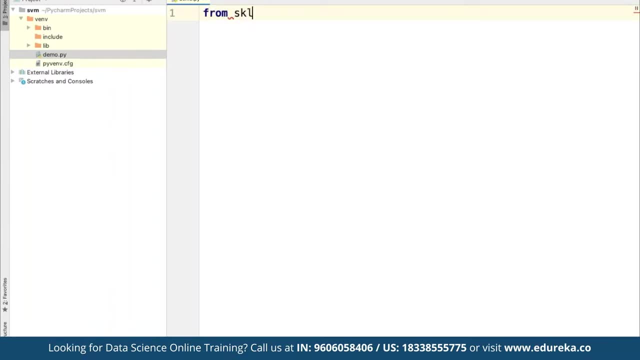 So first of all we are going to work from the sklan library, so here we can use. from sklearn we are going to import the data set, so they they are some sample data set available under sklearn Library cells, so here we can define the cancer data set already available under escala and here we can use. 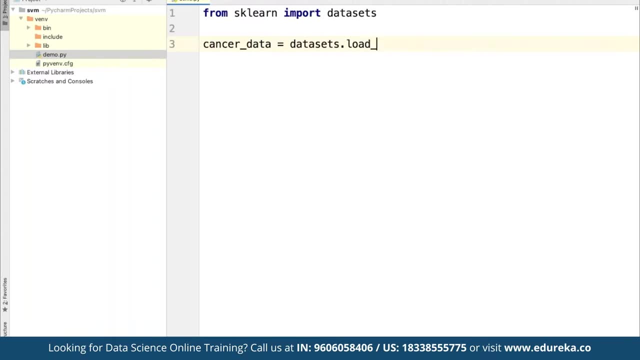 data sets, dot load, and then we are simply going to load support for breast cancer. we can load this current data set already available and now, if we want to simply print the current data set that we can, that we have currently imported. so here we can find cancer data, dot data, and again, we only want 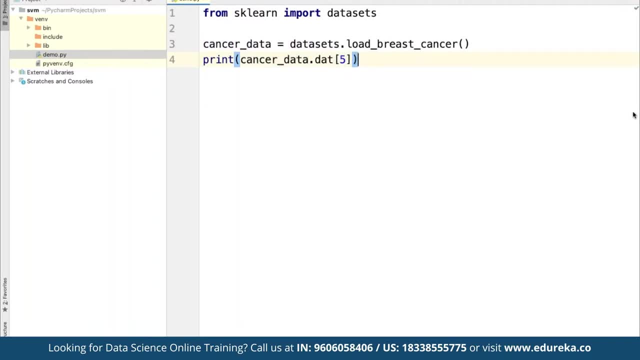 to print the five first rows available in that. so here we can define these statements here. so we have. we are going to use a sample data set currently available and whenever we are going to work on any project, in case they are now, in case the data set is not available, then we can go ahead and simply. 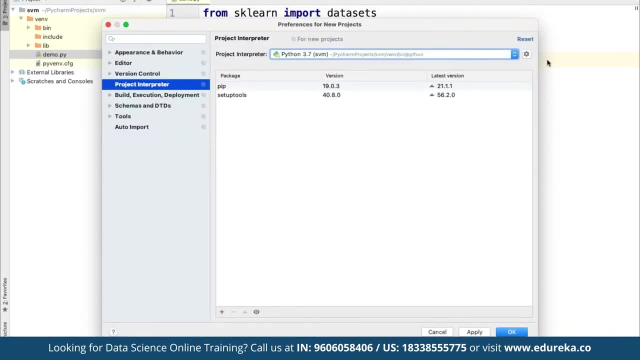 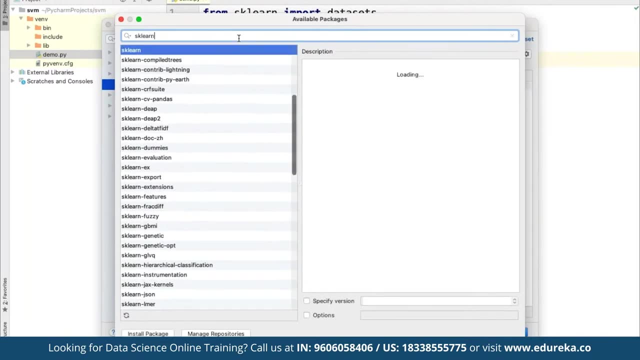 install more libraries by simply choosing the current data set and then here we can go ahead and click on add and from here we can search for any bibli. that is that we that may be missing. for example, here we are going to work on escalant, so we have to make sure that we do import escalant, because without escape library 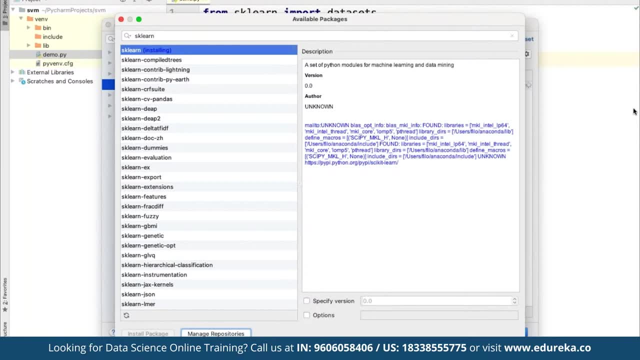 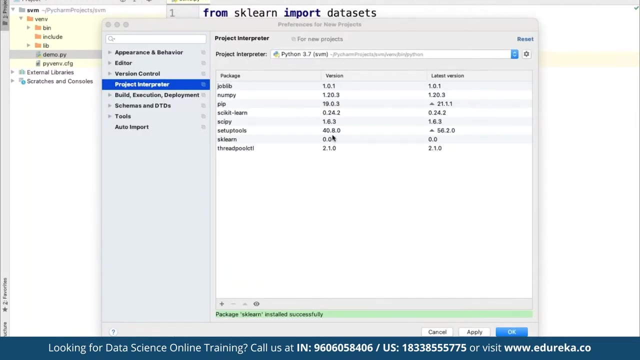 we will not be able to work on the spm here, so here we are simply going to work on the sample data set. all right, so, as you can see, now escalant has been installed. so again, this is a. this is a packet that we're going to work with, so here we can close it if we want to. 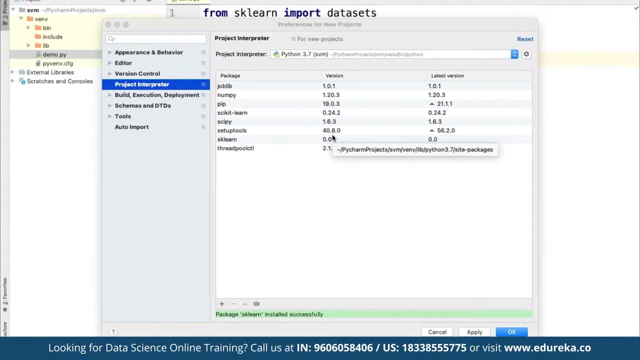 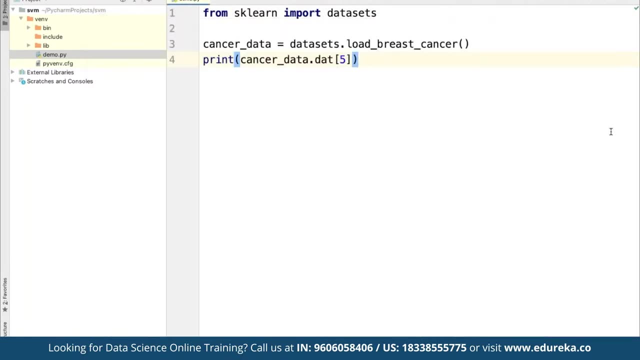 work on the other components, we can search for any library and then we can have it installed. all right, so now we can click on apply and then once we top- because if we don't have the library installed and then if we try to turn this up, it will simply go to throw us an error and, as 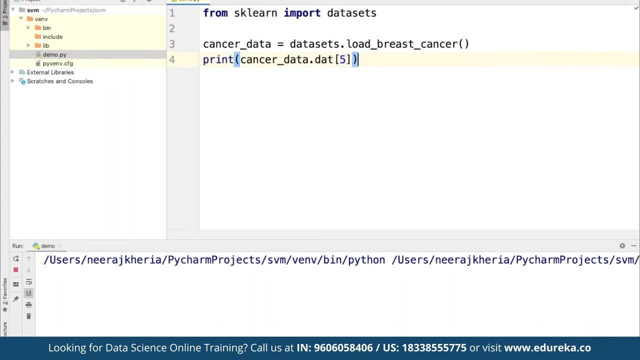 you can see, currently this is going to update the package and then from there it is simply going to load the breast cancer relationship, which is available as an inbuilt sample in SQL. so it is simply going to get connected to the server and then from there it is going to be going to pull the load, the breast. 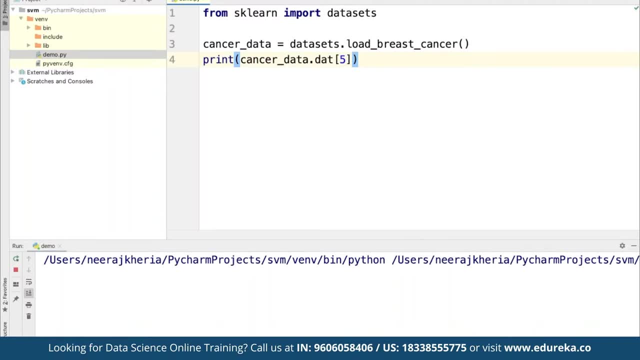 cancer leader said, and then it is simply go to print the first five rows from that data set. so it may take a while, depending upon how, which data set we have imported. so before we perform any calculation, let me just show you how started this looks like. again in the meantime, this is getting pulled here. so 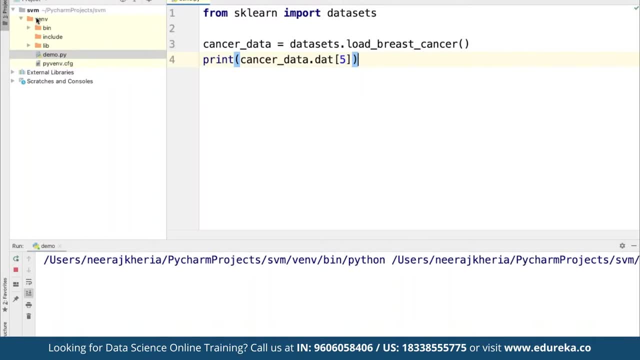 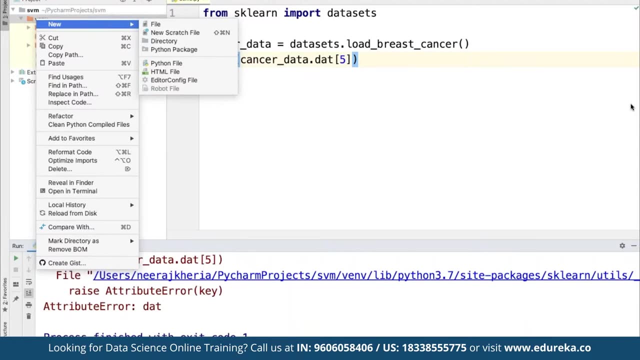 we can simply go ahead and create a new file. it has been timed out because of memory error. okay, we define, we misspell data. it has to be the data itself. that only doesn't be going to. so, as you can see here, now we have the first five rows in. 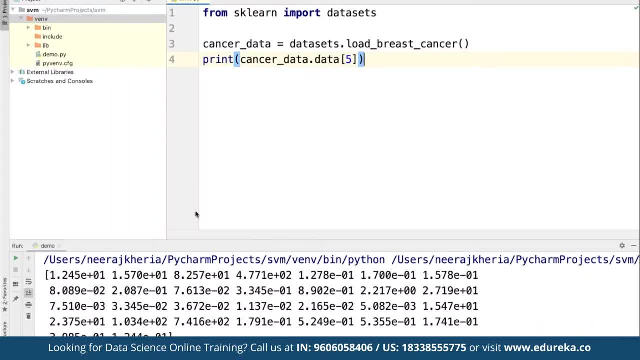 terms of this breast cancer data, which has been pulled automatically from SQL, as you can see here, right so now, we are going to define the data set. right so now. if we are going to simply split the data, right so, we are simply going to divide the data into trading set and the test set to. 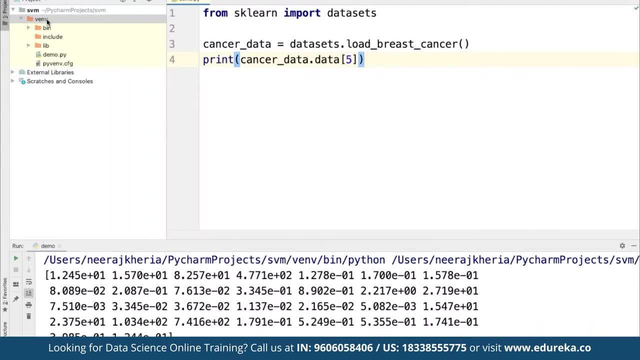 get accurate results, and after this we will spread the data using a train test split function. so here we are going to need three parameters, like in the example that we have that we are going to see. so from here we are going to load the current data set. so, for example, not here now, just to avoid confusion, for 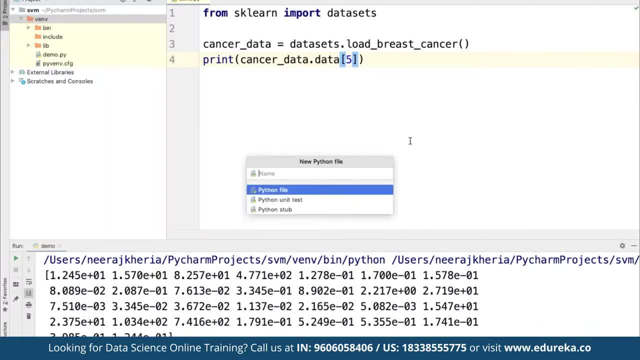 yours, so we can create a new file. let's say, we define sense as, suppose, number two, so here we can define from sklearn. so first of all we define from sklearn library, from sklearn dot model, and here we can define model selection. so here we are going to import train test split, as we discussed. 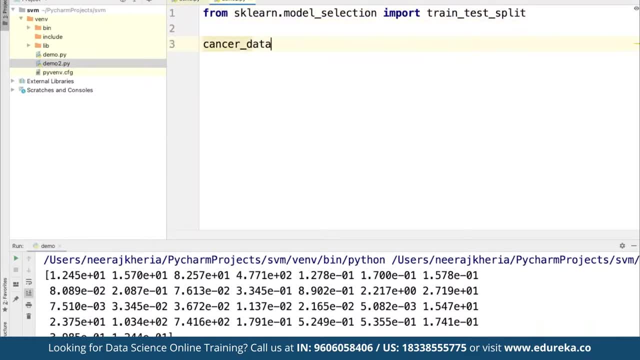 we are going to split it and then we can define from cancer data that we are going to import. so here we are going to find data set dot load, rest, cancer, which is already available, and then we are simply going to define the models in terms of: suppose here we define x train. 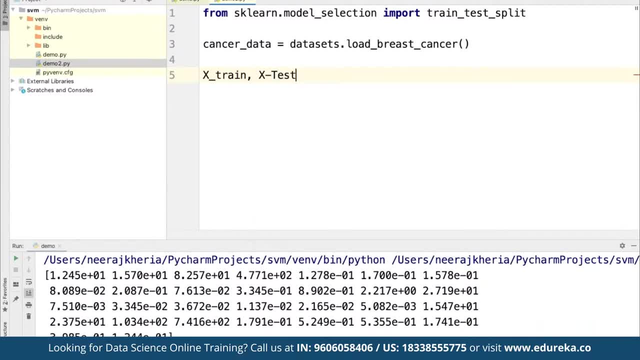 and then we can find x split we can define for x test, and then we can define same thing for y train, for y test, x train, x test, y train, y test. so here we are going to define this from the same train test split that we are going to import, and then here we are going to divide them under: 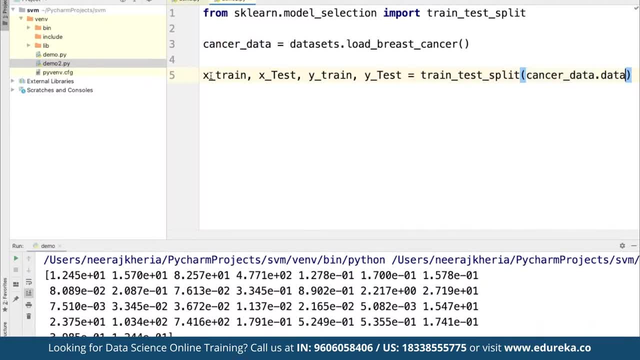 from the cancer data and the data which has been imported here, and then we are going to define this for cancer target. so let's say, here we can define this for cancer data, dot target, and then we can define the test size. here we're going to define the test size. suppose we want to keep the test? 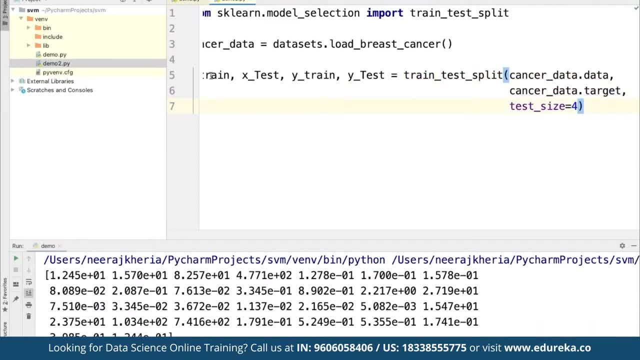 size, suppose as four, let's test has four and then we're gonna find random state. we can define random state, pose one or nine, anything that we want to have. so here we are simply going to split the data set with the given in the X train, X, X test and divide rate and Y. 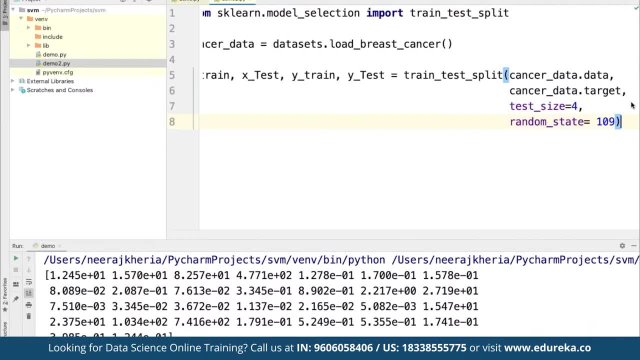 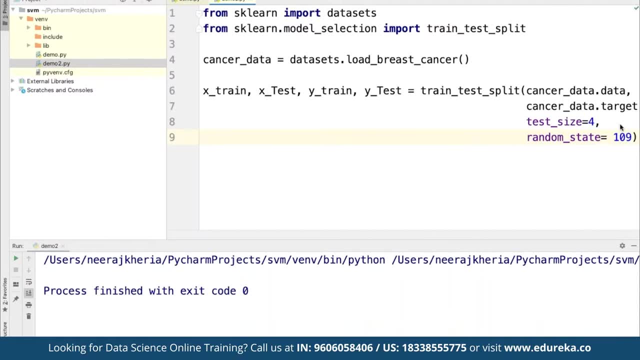 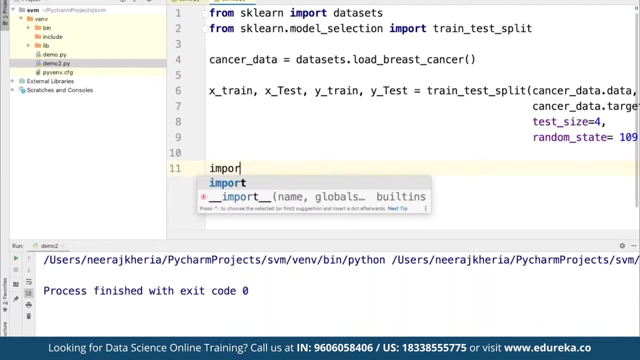 test here. so here the entire set is simply going to be split. so now we are going to generate the model as well. so what we can do. so now here we are going to check. we can say generally bottle, and for that we can import on a library for. 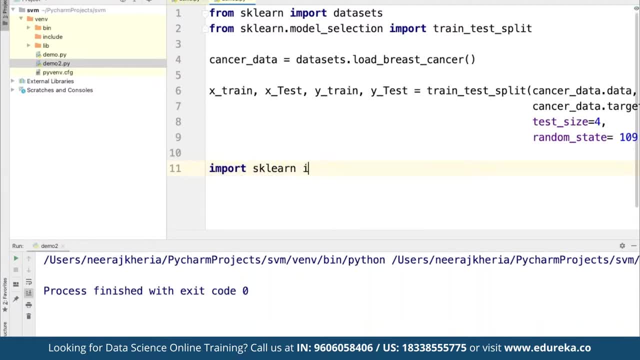 example, here we can import, let's say, a scalar and here from a scale and we are going to import the SVM. so here we are going to create the library. so here we could create a classifier here. so first of all we're gonna find classifier as opposed SVM, dot, SVC, and here we can find the kernel, here we can find the kernel. 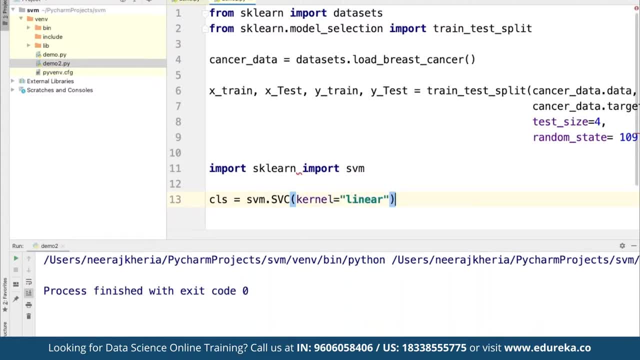 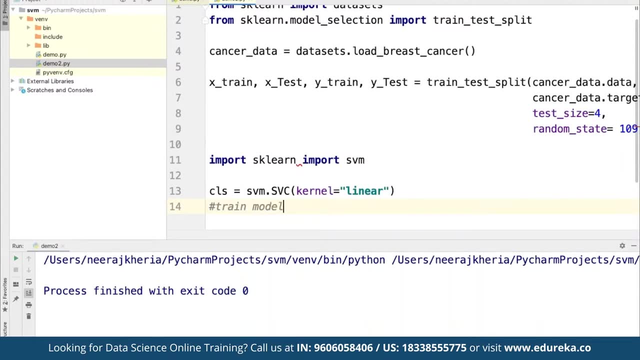 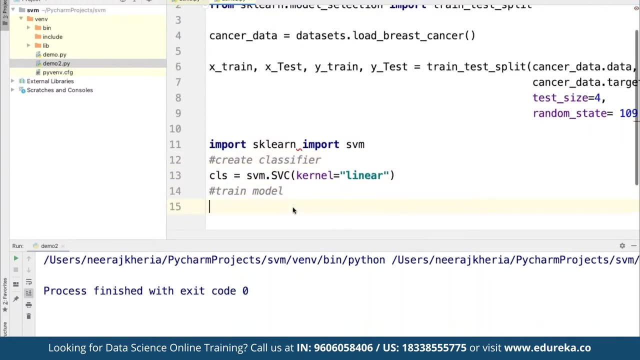 I suppose linear, whatever you want to call it to use- we can define that. and then we are going to train the model. so we can say: we are simply going to now train model. so here we have create classifier and now we are going to train the models. so for training one, we can define class. 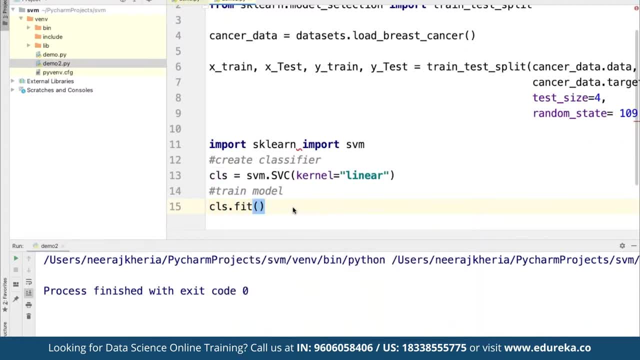 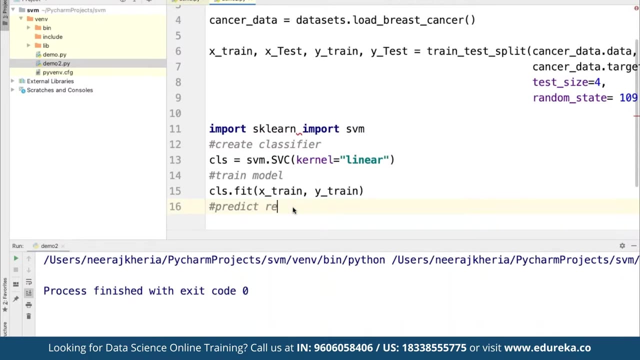 dot fit, and then we can define this value as X train that we have already imported, and then we can define for Y train that have we have already performed the split on, and then simply we are going to have a prediction done. so here we can define predict response and for getting the response we can define prediction as: 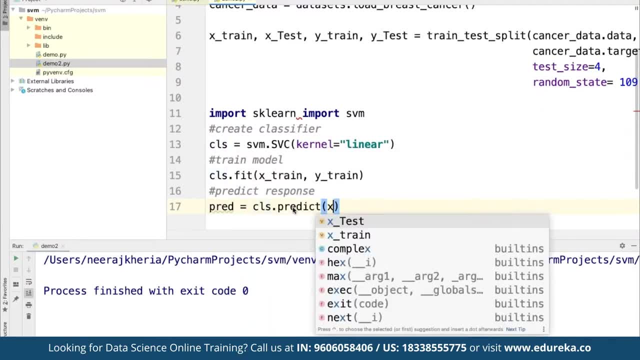 class dot, predict, and for this we are going to make use of X test that we have already defined. we define for X train and for Y train and then for prediction we are simply going to do that on the text on the X underscore test that we already have defined. 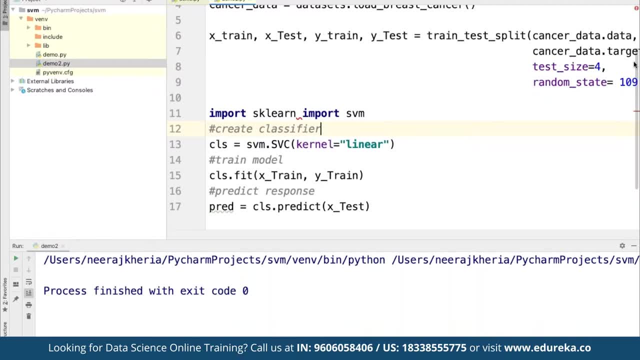 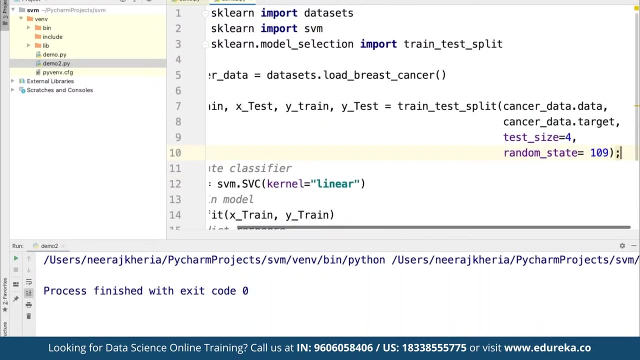 that depends upon type of data that we have. so that totally depends upon the type of data we are going to simply import and let's move this import from the end up here. so you have to define this. in the top section is up from escalon. we are simply going to import the SVM. if we had to find all right and 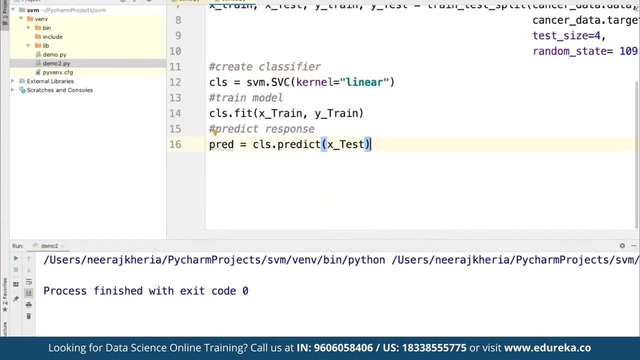 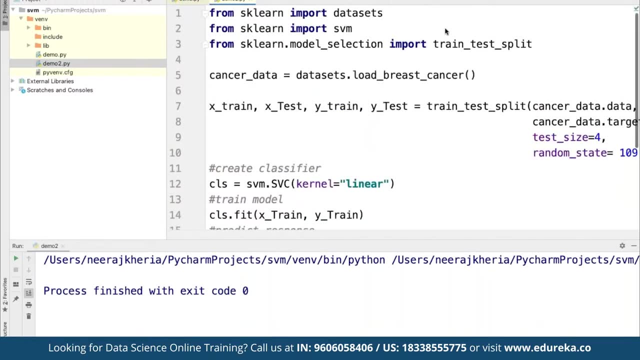 now we had to find a classifier. now we are going to evaluate the model, and for evaluating the model we can simply go ahead and define. so here, from a scalar we can also import other components as well. from escalon, we are also going to import metrics, so here we are also going to 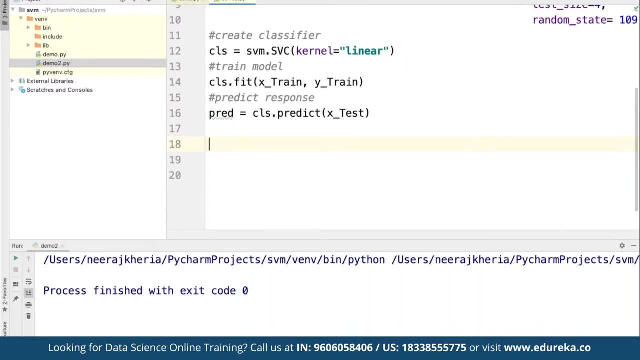 import metric and by using macro accuracy metric for getting the accuracy we can find. for getting the accuracy we are going to define, we are simply going to print the accuracy of the prediction here. and for accuracy, we are simply going to define metrics, which is again available under the metrics that we have, we have accuracy. 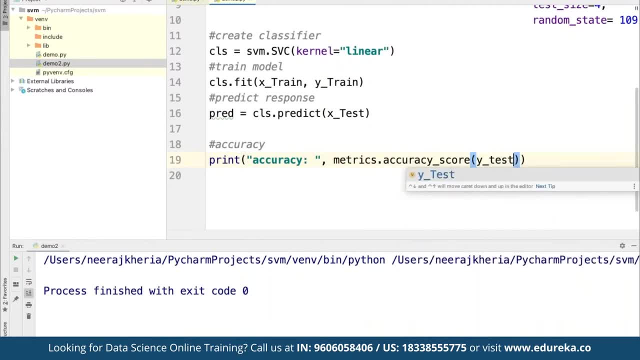 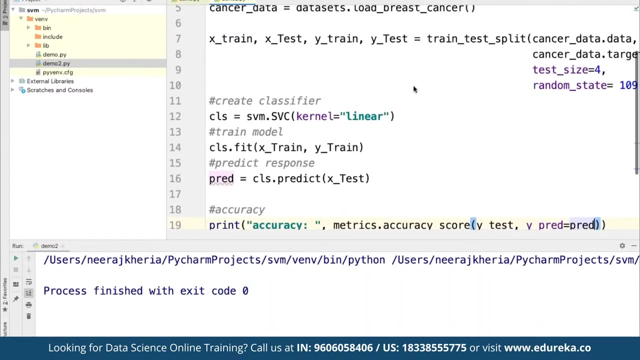 score and then from here we are simply going to find why test and we are going to finance before why prediction as well, that we have defined. so I think we have used why test, we have used a per case for, for we have used. let's do one thing. 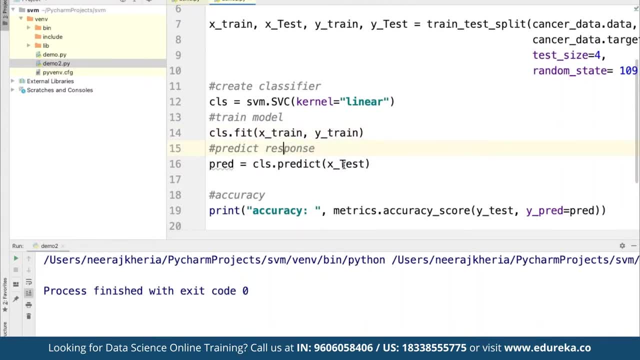 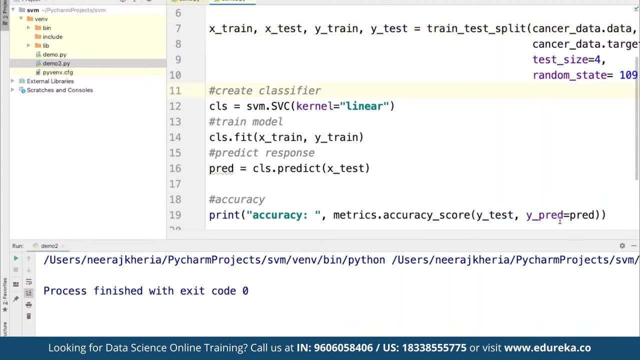 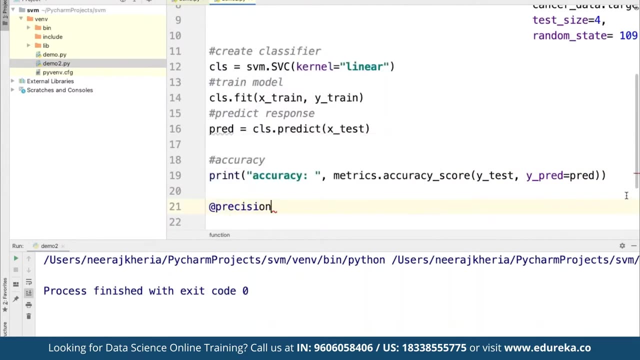 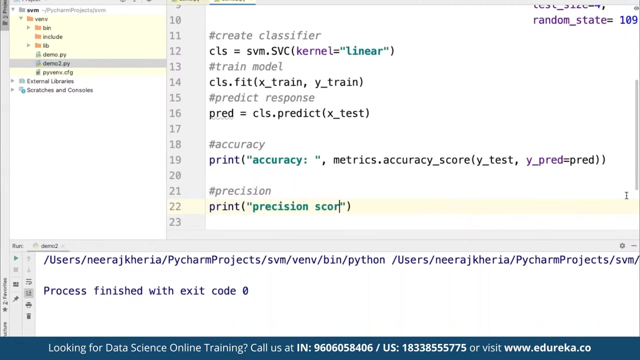 let's use small case for everything, just to avoid confusion, as it finds us test, train and test again. so you have your y test and then you depend here. we define it for production and then for finding the precision score. for finding precision, we can simply print another statement as precision score. 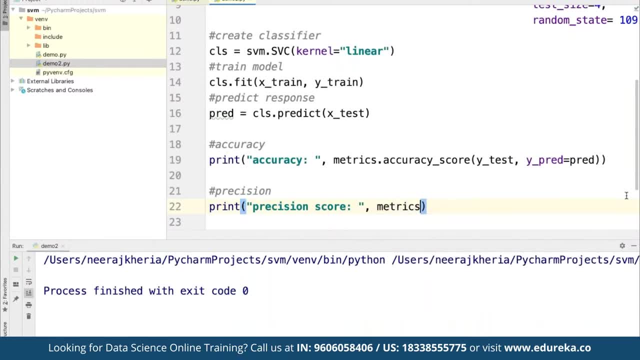 and in here we can again make use of metrics, and for metrics we can define the precision score itself. so here we can define precision underscore score, and in here, for precision score, we are going to make use of y test, and then we are going to make use of y prediction. 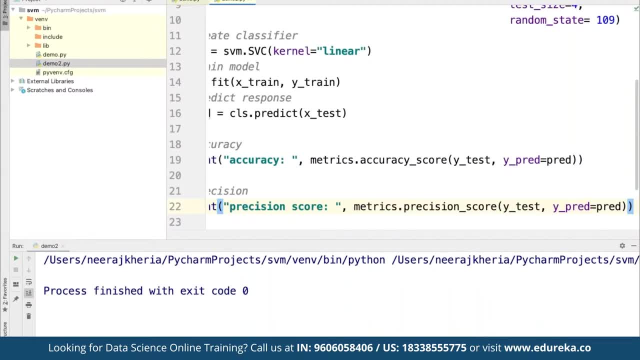 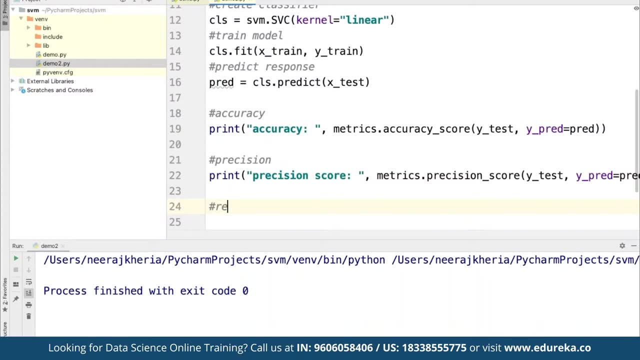 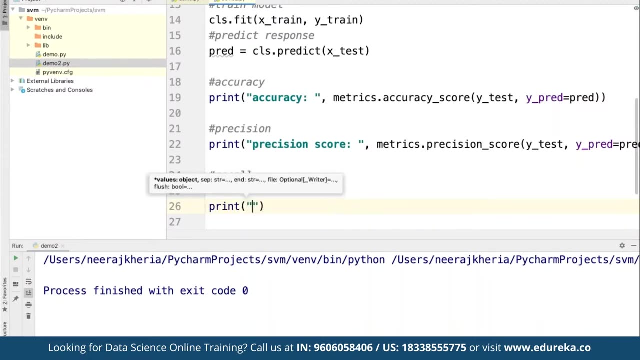 all right. and then at the end, if you are simply going to recall the score and we are simply going to report, so here we can define for us that i want to call mark. we can print another statement for recall. we can call this as recall. we can print another statement for recall. we can define this one as: 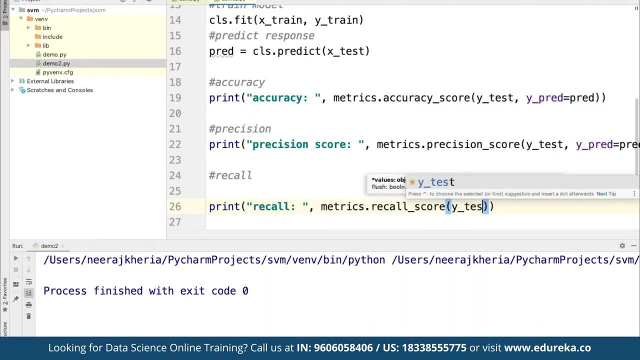 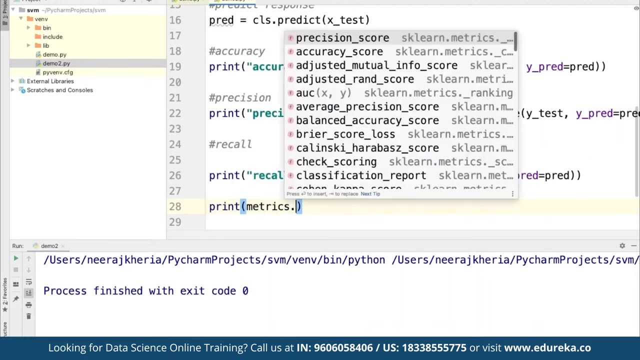 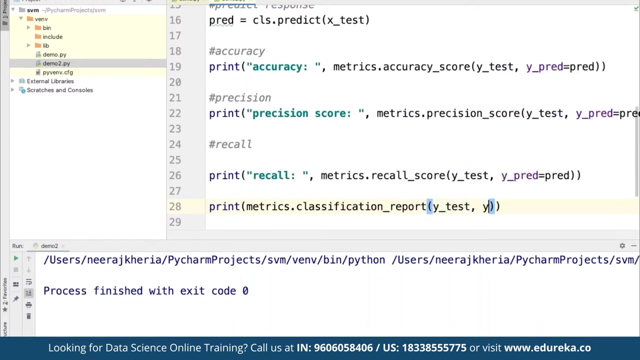 recall and here from save metrics dot recall score and for here we can define y test and y prediction andb y. if you want to print all the metrics, so here we can find print metrics dot classification report and for that we are going to make use of y test and y prediction for prediction made. all right. 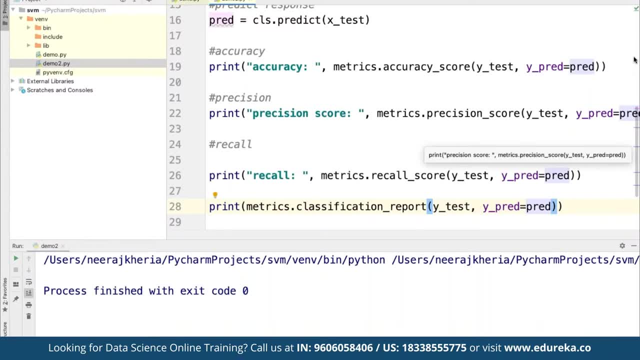 so here we had to find these, and now, once we have configured everything, so here we can simply run this up and we would be able to see the entire output which, once it has been defined, so now we can see. here we have the accuracy, here we have the precision score, the recall score that we have. 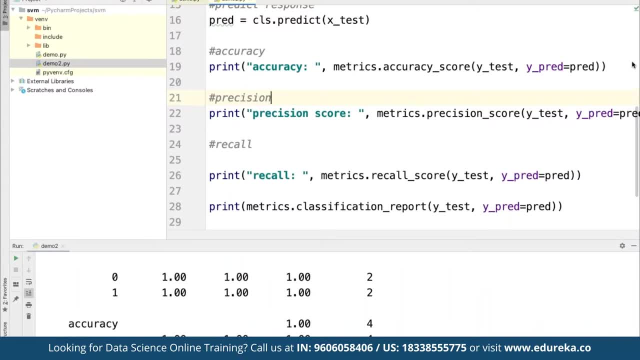 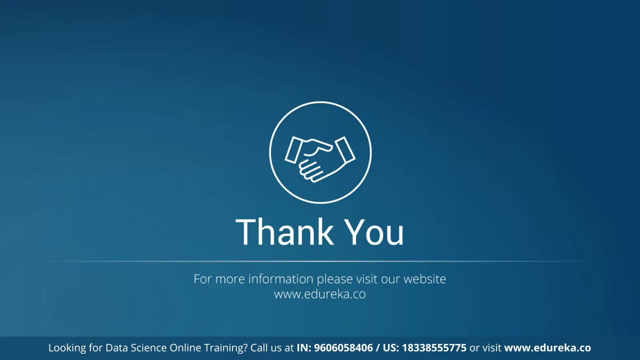 defined, and then we define the accuracy based on whatever data we are going to work on. depending upon that, we are simply define the current data set here. thank you so much for joining guys, and have a great day. take care, bye, bye, you, you, you.